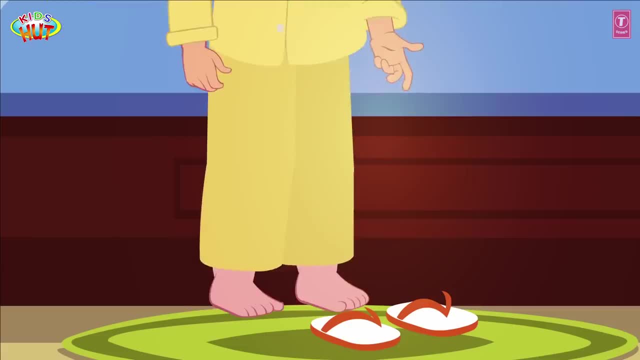 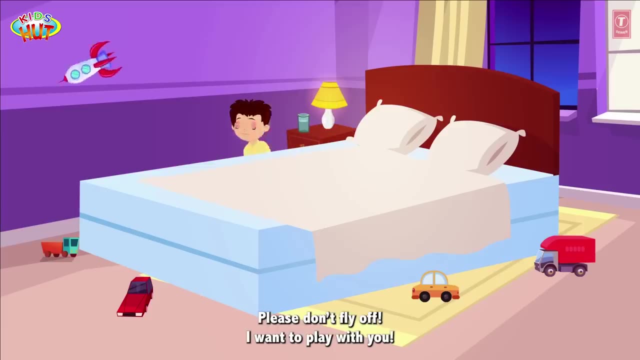 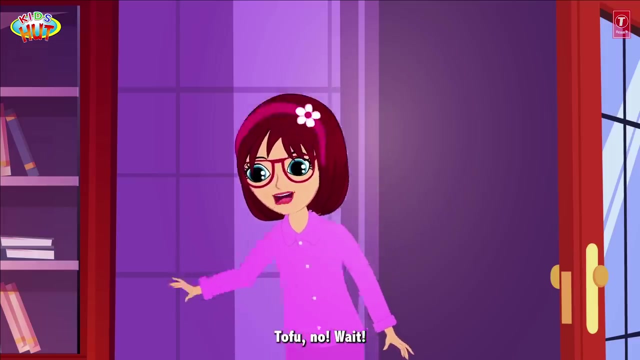 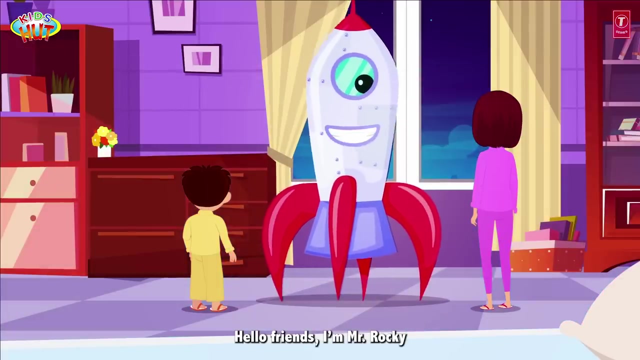 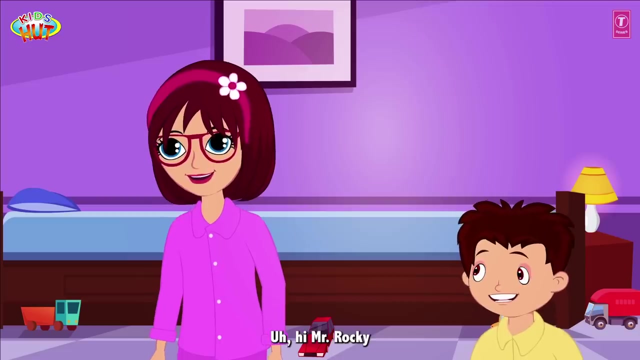 Tofu. what is this noise? Will you stop playing, please? I can't sleep. Please don't fly off. I want to play with you, Tofu. no Wait, Hello friends, I am Mr Rocky. I'll take you to the space today. come sit inside. uh hi, mr rocky, whoa easy. 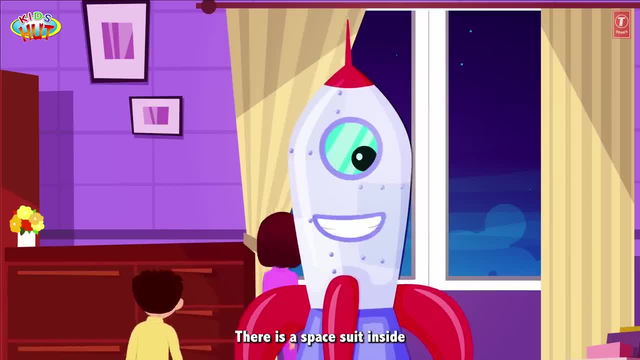 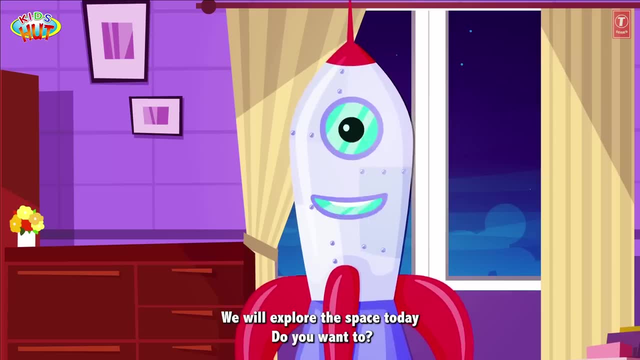 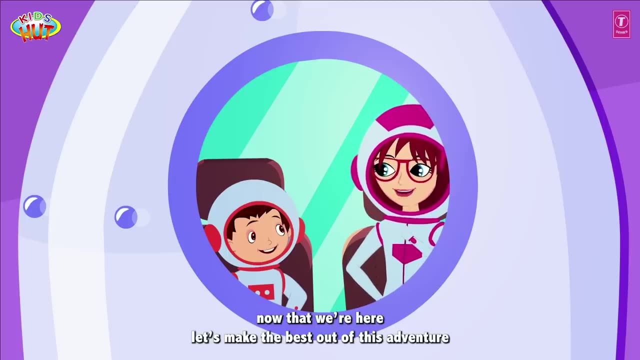 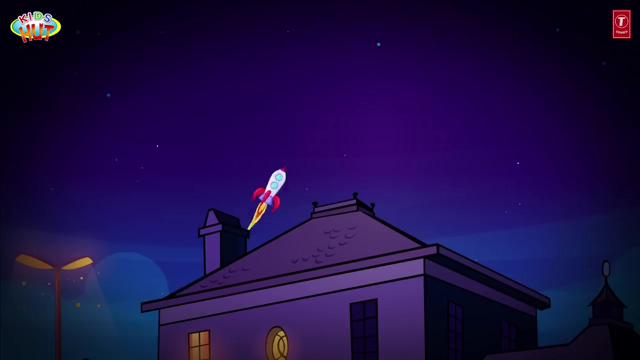 Tia, wait for me. there is a spacesuit inside. wear it, please. we will explore the space today. do you want to? oh, yes, I would love to. yeah, now that we're here, let's make the best out of this adventure awesome. I will show you some. 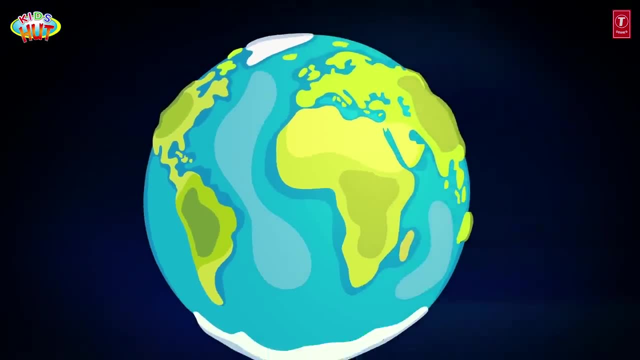 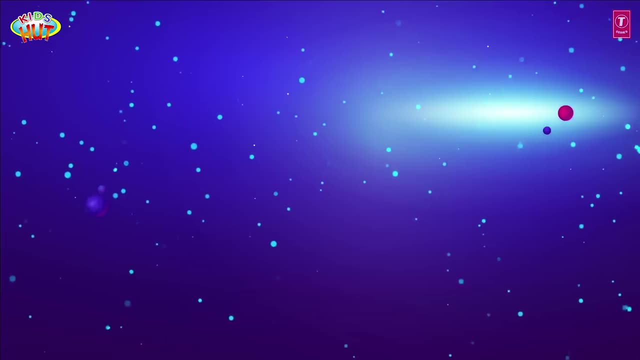 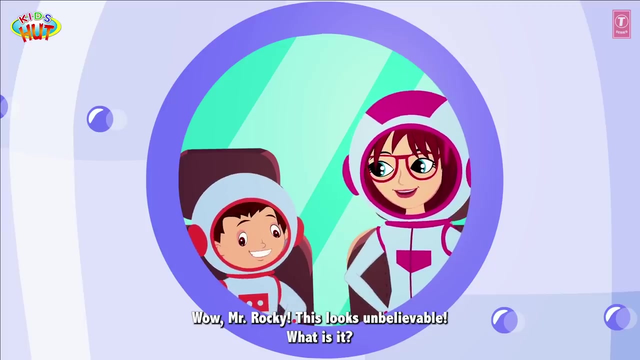 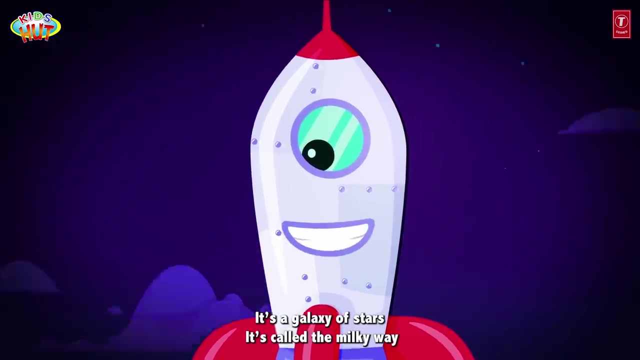 amazing things out there. look, we just left earth. Wow, isn't it beautiful? indeed it is. Wow, mr rocky, this looks unbelievable. what a beautiful space it is. I'm so excited to explore the space with you. what is it? it's a galaxy of stars. it's called the Milky Way tofu. look, it's the. 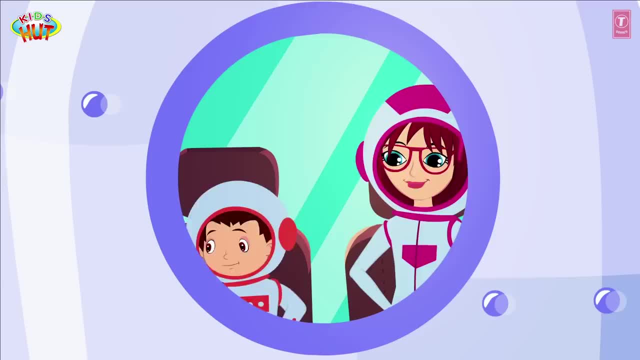 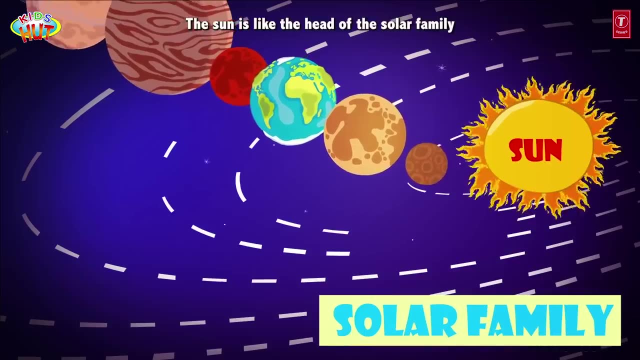 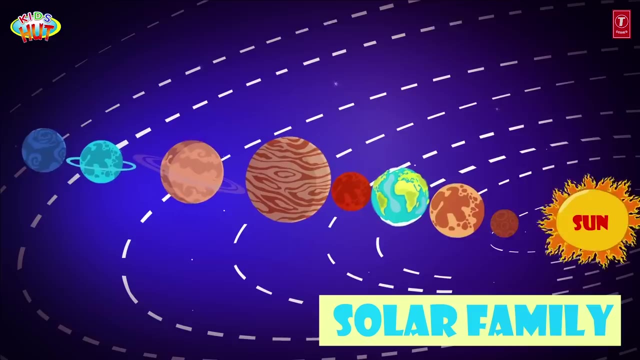 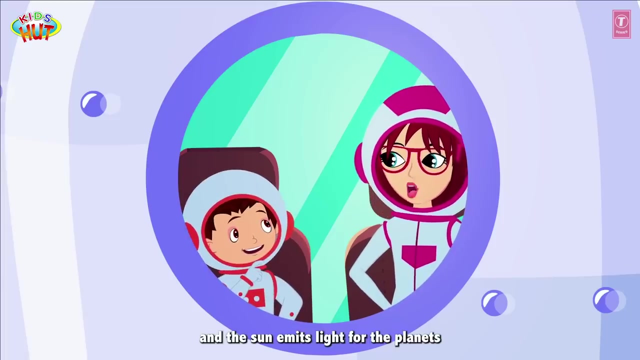 solar system. uh, what's that? it's a collection of eight planets. the Sun is like the head of the solar family. but why is the Sun the head of the solar family? because all the planets need light to survive and the Sun emits light for the planets. all the planets revolve around the Sun. 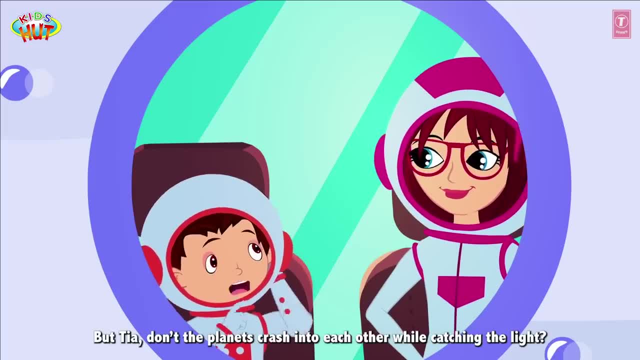 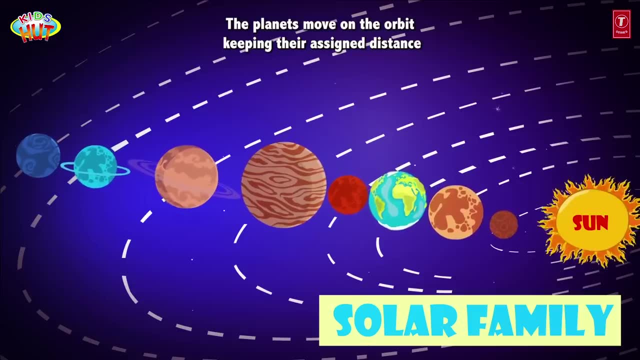 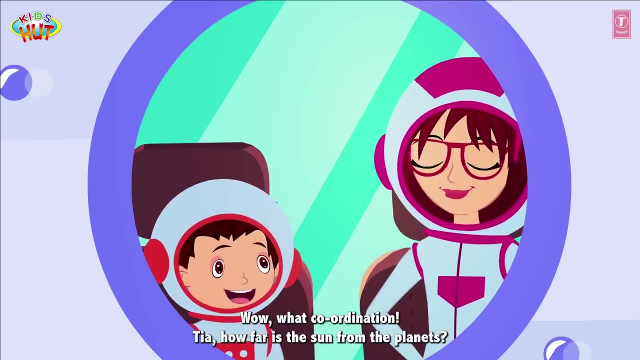 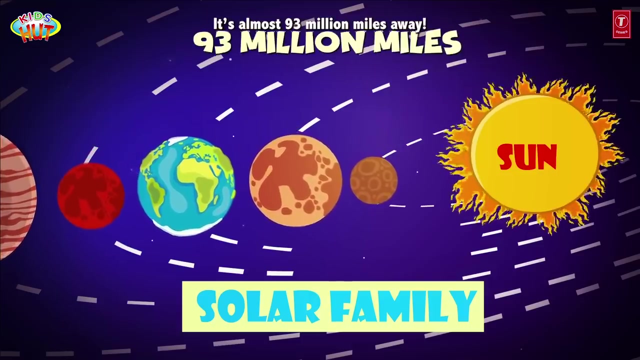 for light, but, Tia, don't. the planets crash into each other while catching the light, no tofu. the planets move on the orbit, keeping their assigned distance. wow, what coordination, Tia. how far is the Sun from the planet's it's? It's almost 93 million miles away. 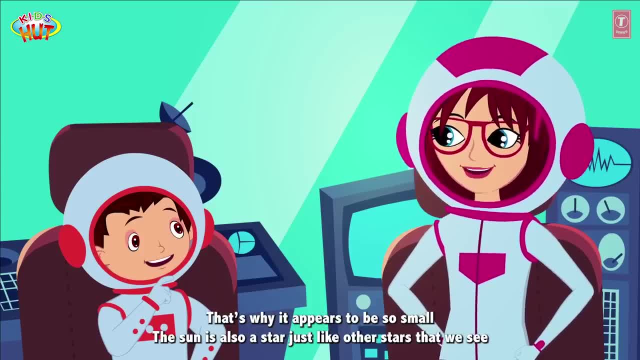 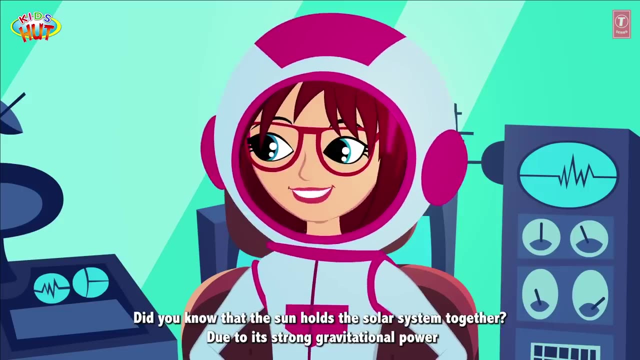 That's why it appears to be so small. The Sun is also a star, just like other stars that we see. It's the biggest object in the solar system. Wow, I didn't know that. Did you know that the Sun holds the solar system together? 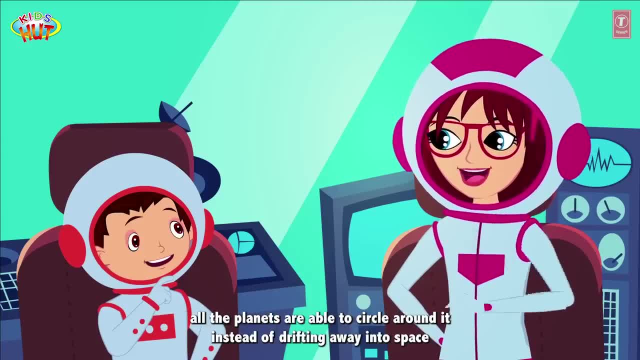 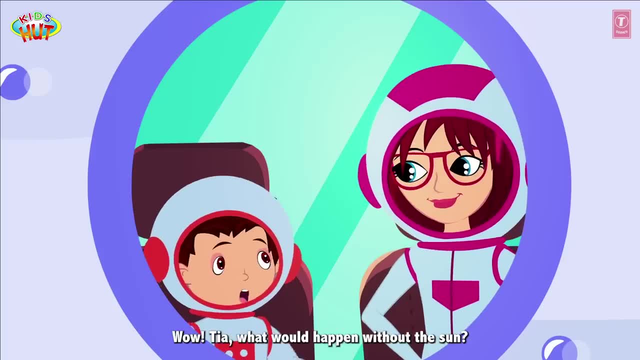 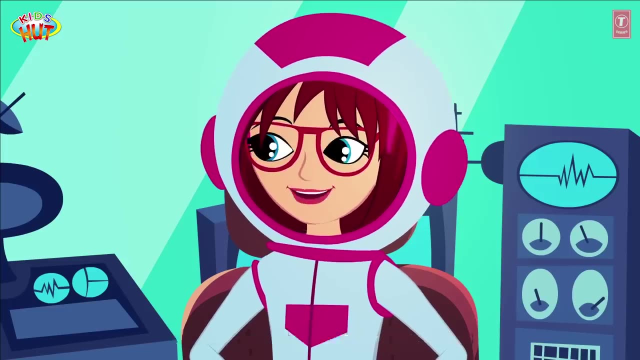 Due to its strong gravitational power, all the planets are able to circle around it instead of drifting away into space. Wow, Tia, What would happen without the Sun? Without the Sun, there would be no light or heat, Even the water would freeze and nothing could survive. 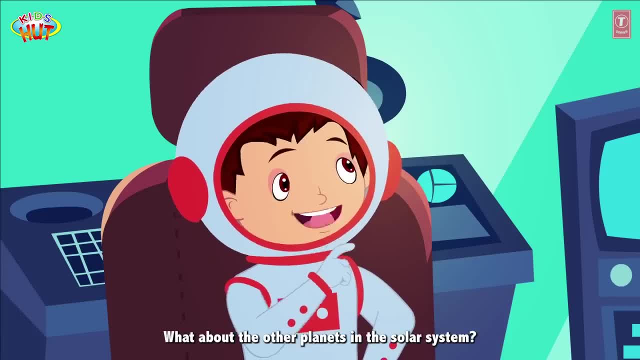 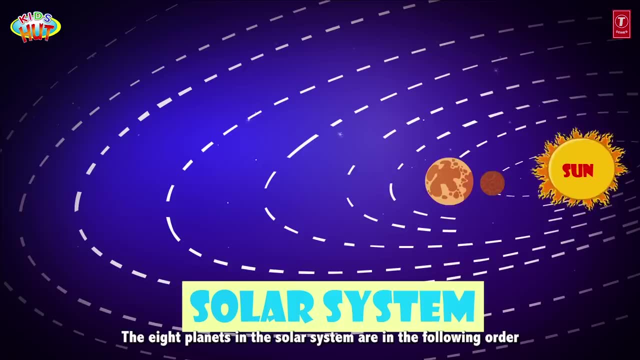 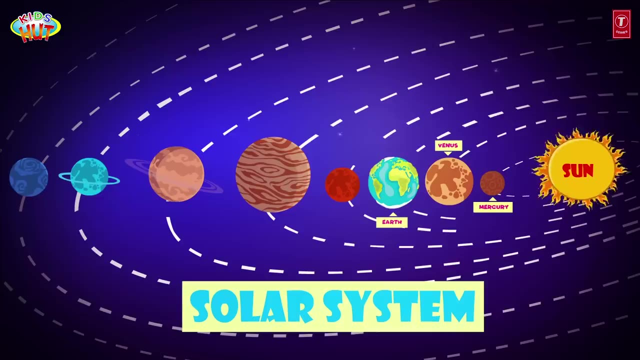 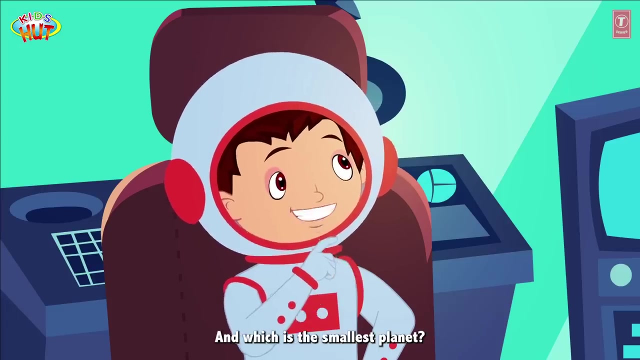 The trees would die too. What about the other planets in the solar system? The eight planets in the solar system are in the solar system. They are in the following order: Mercury, Venus, Earth, Mars, Jupiter, Saturn, Uranus and Neptune. And which is the smallest planet? 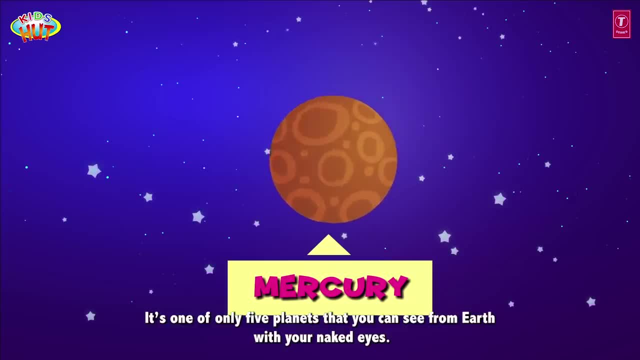 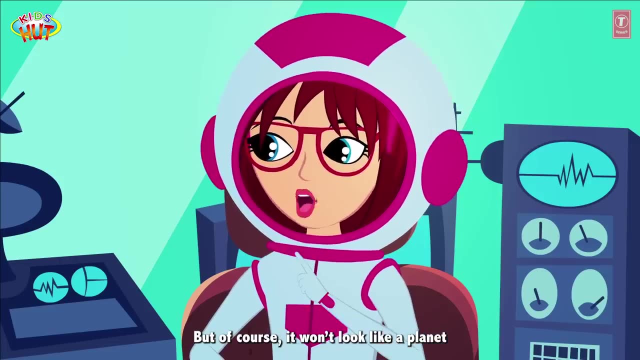 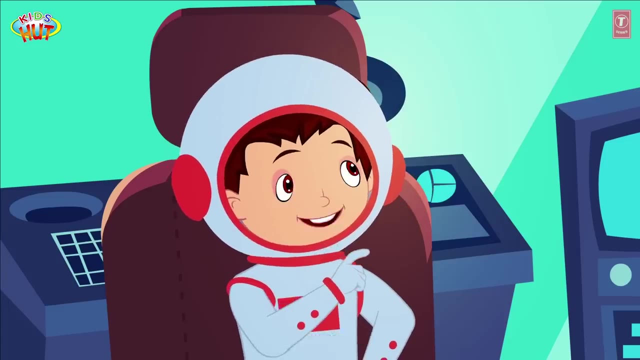 It's Mercury. It's one of the only five planets that you can see from Earth with your naked eyes, But of course it won't look like a planet. It looks like a bright star when you see it from Earth. That's amazing. 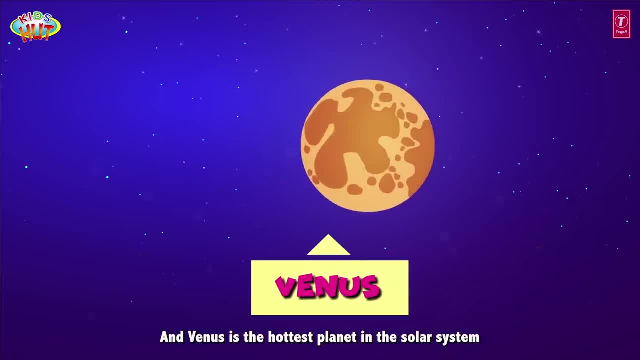 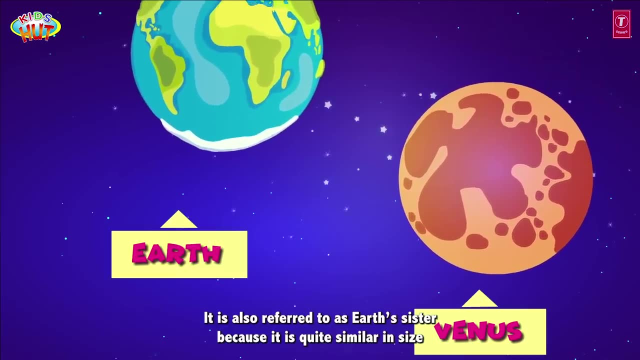 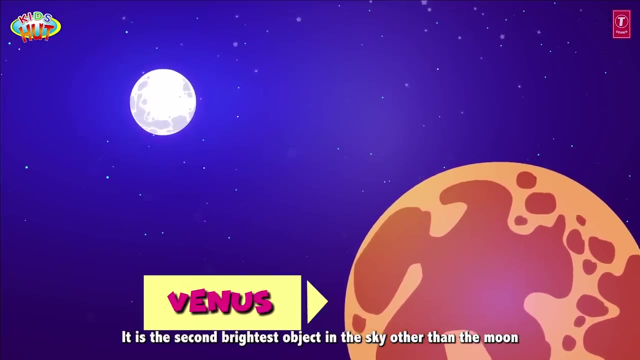 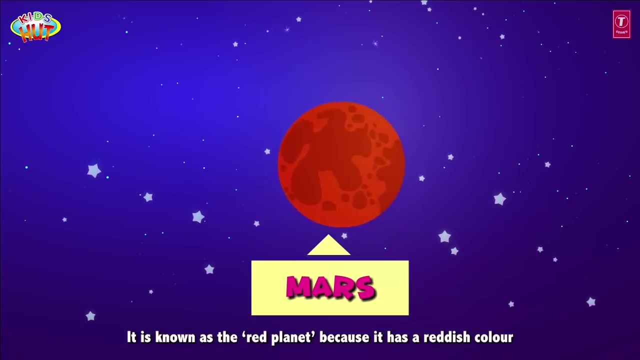 And Venus is the hottest planet in the solar system. It is also referred to as Earth's sister because it's quite similar in size. It is the second brightest object in the sky, other than the Moon. What about Venus? What about Mars? It is known as the red planet because it has a reddish colour. 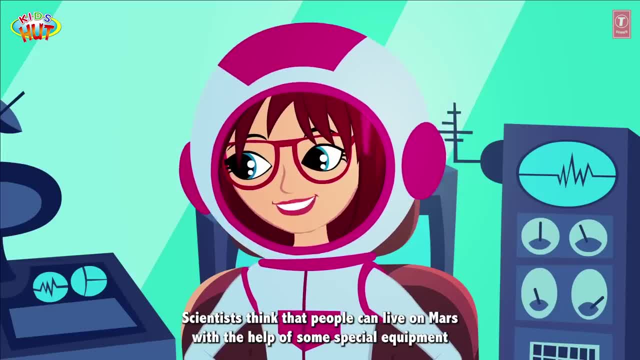 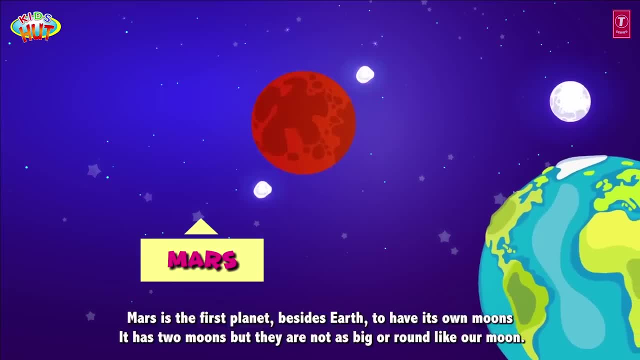 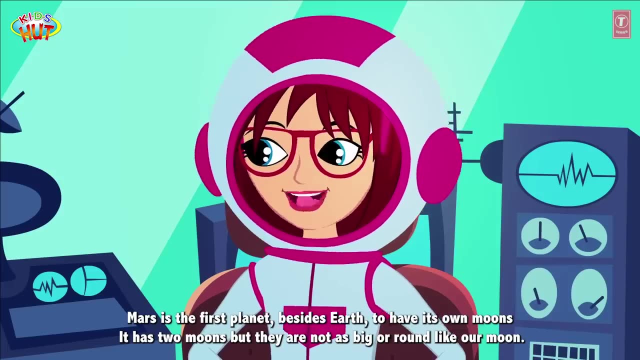 It is cold and rocky. Scientists think that people can live on Mars with the help of some special equipment. Mars is the first planet besides Earth to have its own moons. It has two moons, but they are not as big or round. It has two moons, but they are not as big or round. 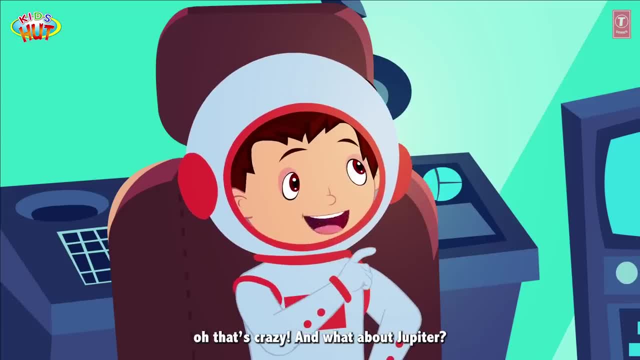 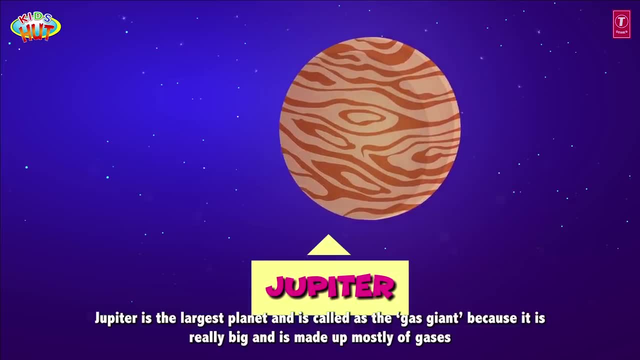 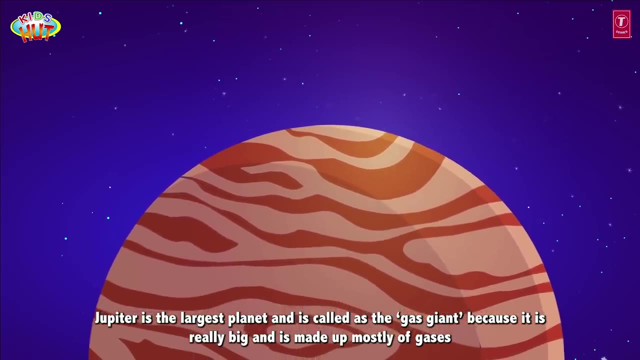 It has two moons, but they are not as big or round. Oh, that's crazy. And what about Jupiter? Jupiter is the largest planet and is called as the gas giant because it is really big and is made up mostly of gases. Then comes Saturn, another gas giant. 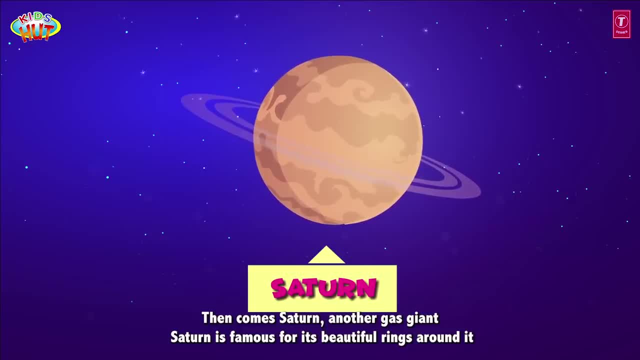 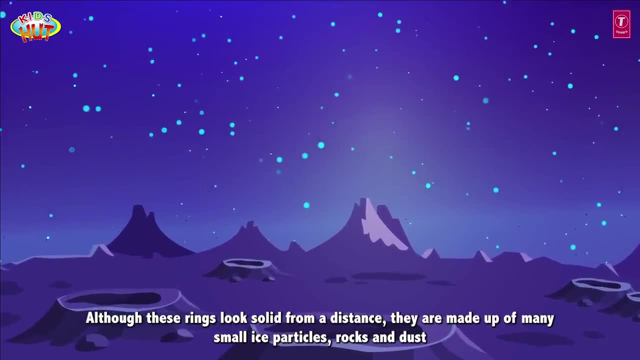 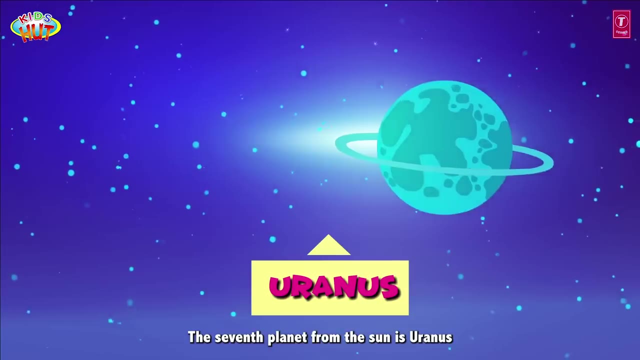 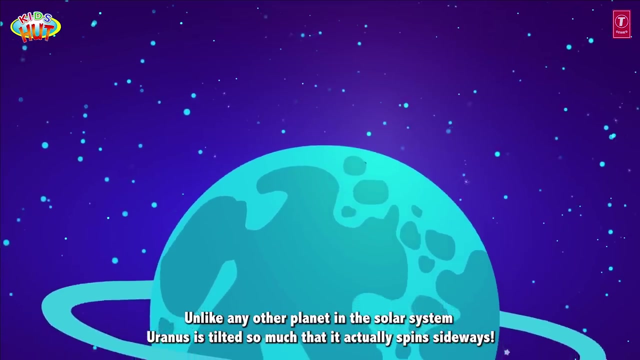 Saturn is famous for its beautiful rings around it. Although these rings look solid from a distance, they are made up of many small ice particles, rocks and dust. The seventh planet from the Sun is Uranus. Unlike any other planet in the solar system, Uranus is tilted so much that it actually spins sideways. 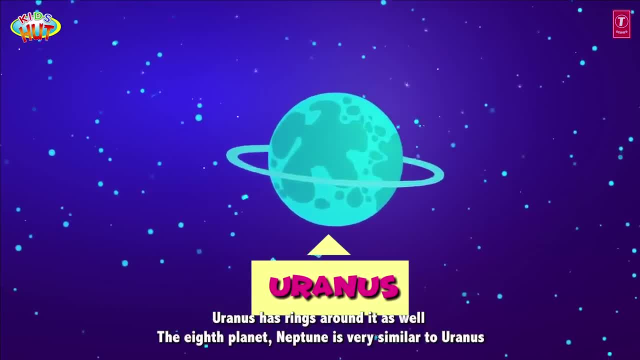 Uranus has rings around it as well. The eighth planet, Neptune, is very similar to Mars. The eighth planet, Neptune, is very similar to Mars. The eighth planet, Neptune, is very similar to Mars. The ninth planet, Neptune, is very similar to Uranus. 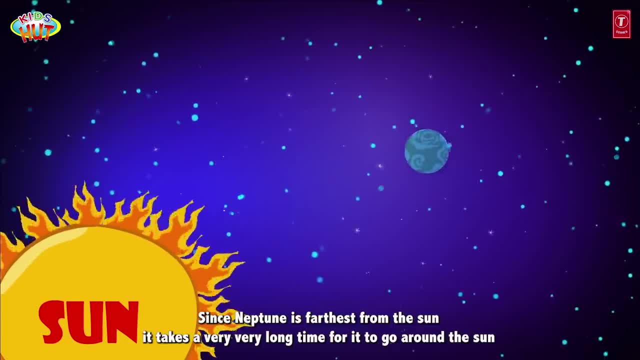 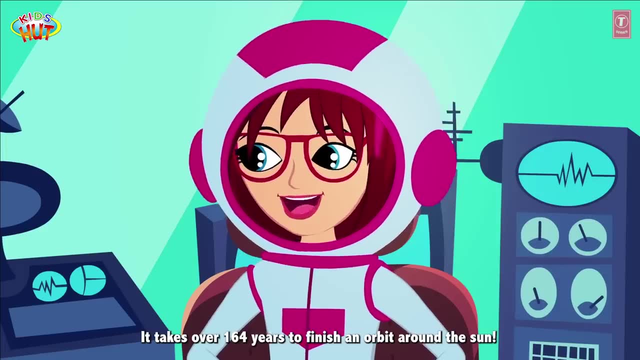 Since Neptune is farthest from the Sun, it takes a very, very long time for it to go around the Sun. Since Neptune is farthest from the Sun, it takes a very, very long time for it to go around the Sun. It takes over 164 years to finish an orbit around the Sun. 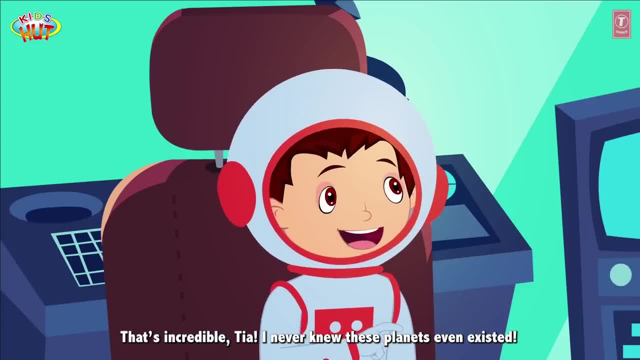 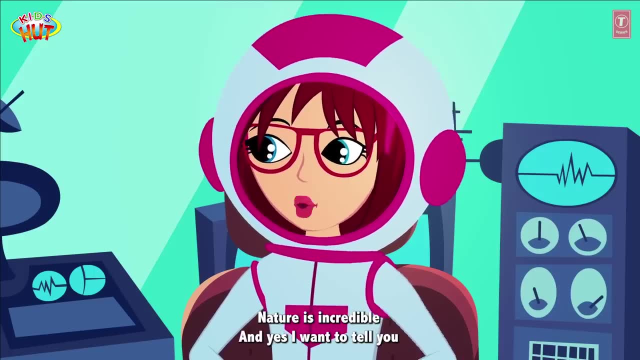 That's incredible, Tia. I never knew these planets even existed. Nature is incredible. And yes, I want to tell you that there was a ninth planet in the solar system. And yes, I want to tell you that there was a ninth planet in the solar system. 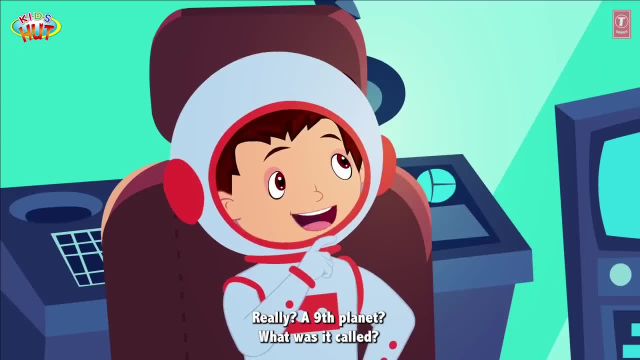 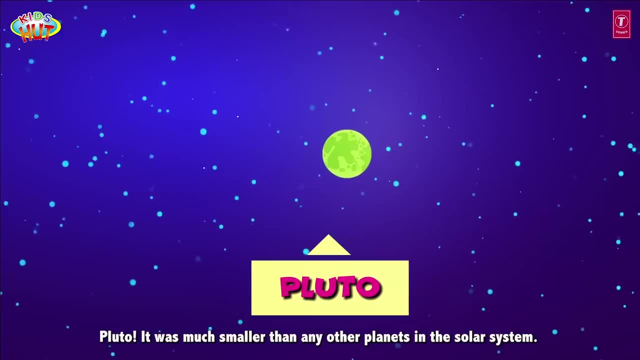 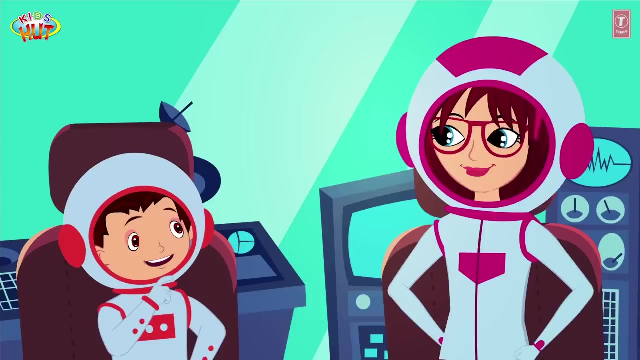 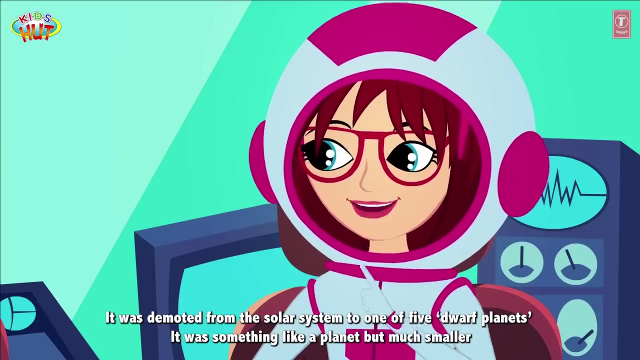 ninth planet too in the solar system. really a ninth planet. what was it called Pluto? it was much smaller than any other planets in the solar system. then what happened to Pluto? it was demoted from the solar system to one of the five dwarf planets. it was something like a planet, but much smaller. that leaves us.